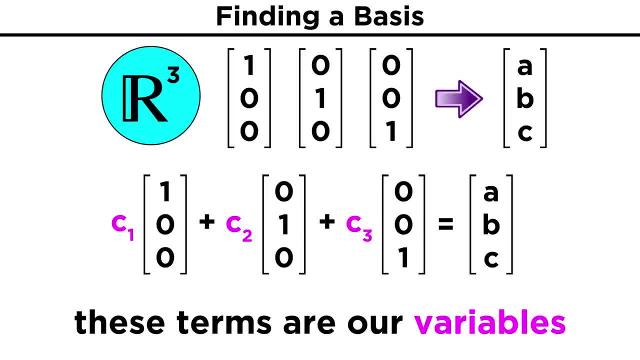 It's important to remember that the scalars we multiply our vectors by which are C1,, C2, and C3, are the variables, while the A, B and C that make up our given vector should be treated as regular numbers on the right-hand side of the equation. 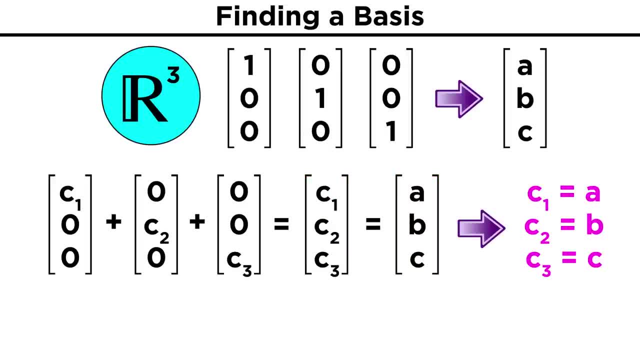 Writing this vector equation out as a system of equations, we get the straightforward result that C1 equals A, C2 equals B and C3 equals C. Because we've found a solution that's possible for any A, B and C. these three vectors spam the vector space R3.. 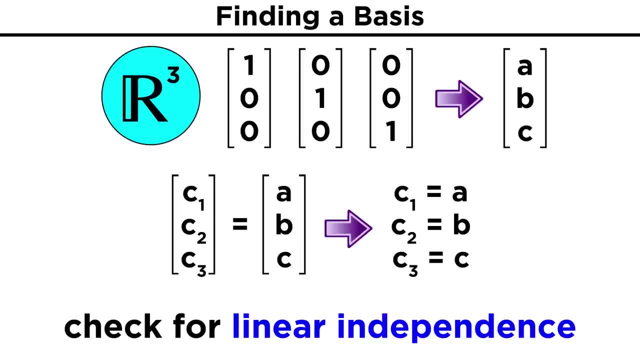 We can easily check that these three vectors are linearly independent by setting the right side equal to zero. So because A, B and C equal zero and, as we saw, C1 equals A, C2 equals B and C3 equals C, these scalars all end up being zero as well. 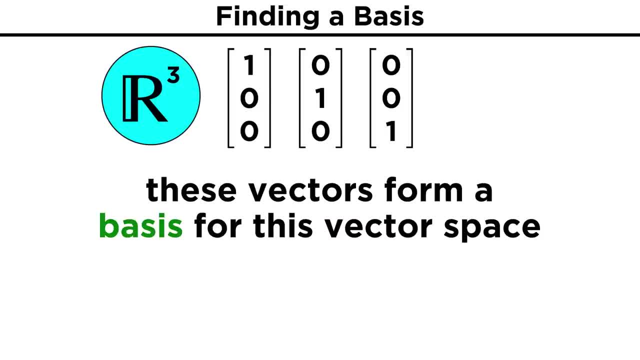 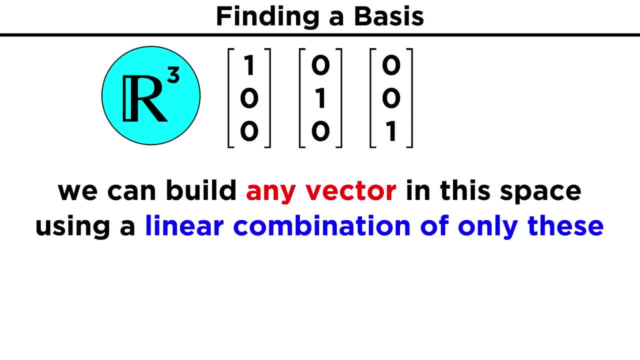 This was our condition for linear independence. It's a very simple solution And we have therefore satisfied the two conditions for these vectors to be considered a basis. They are the building blocks for any vector in R3. And because they are linearly independent, there is no extra information. 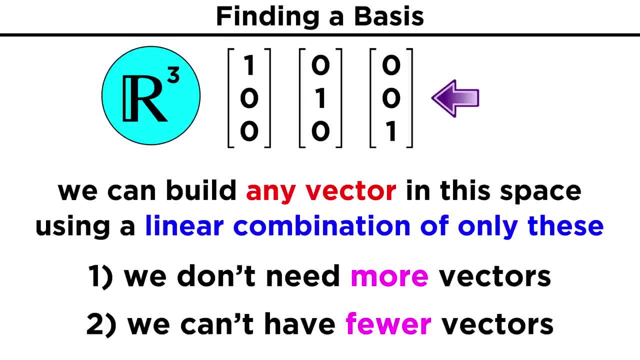 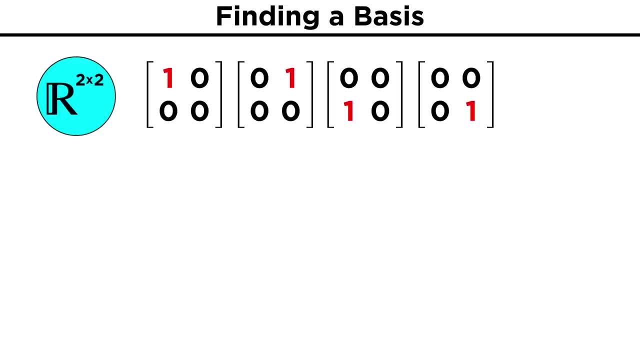 We don't need any more vectors aside from these three, And if we take any away we will no longer span all of R3.. Now let's look at a more complicated example. Let's look at matrices in R2x2.. We could check to make sure. four matrices with a one in each corner is a basis, but 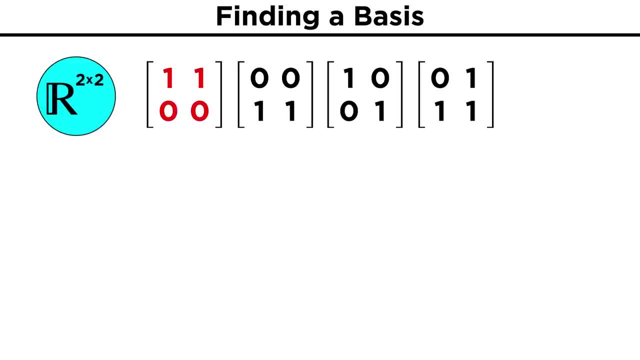 let's instead consider the following four matrices: Ones on the top row with zeros on the bottom, then ones on the bottom row with zeros on the top, then ones on the diagonal with zeros for the other two entries, and then a one everywhere but the top left, which will be zero. 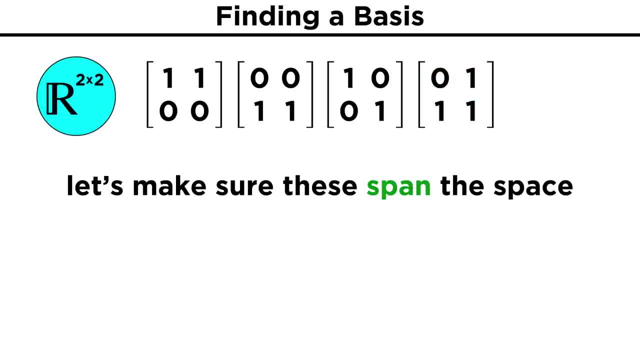 First off, to check that we have zero on the top row. we have zero on the bottom row with zeros on the top. Next off, to check if these four matrices span R2x2,, we will once again set a linear combination of them equal to any given 2x2 matrix, which we can generalize with the entries. 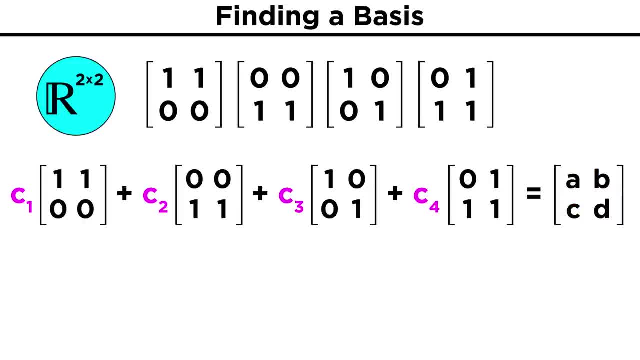 A, B, C and D. So here we have each matrix being multiplied by its respective coefficient and their sum equal to the generalized 2x2 matrix. We can distribute the scalars so that they show up as entries anywhere, And we can also distribute the scalars so that they show up anywhere. 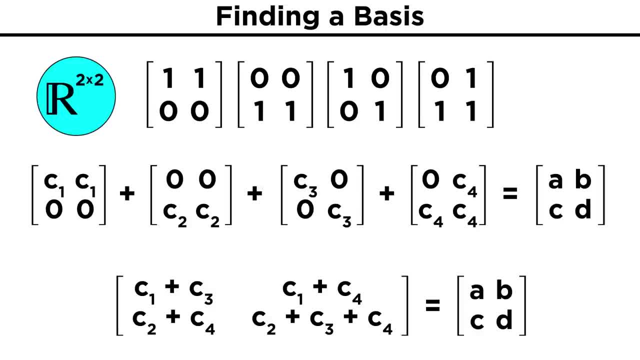 where we had a 1 in a particular matrix, and then we can add up all the matrices to condense things a little bit, and we end up with this new matrix with sums in each of its entries. From here we can write this out as a system of four equations. 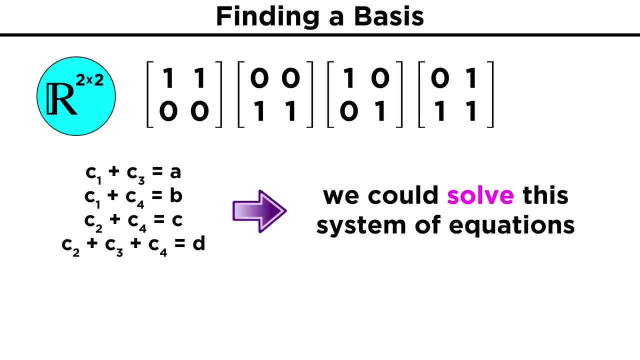 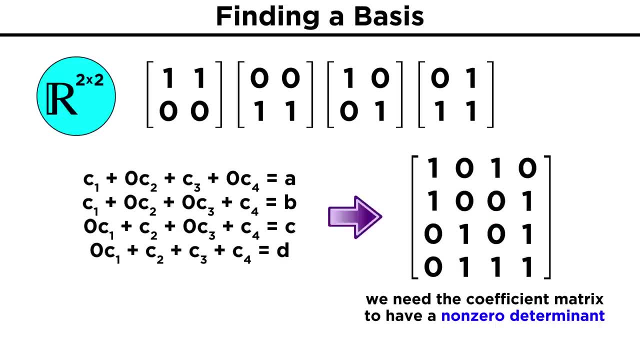 While we could solve this system of equations to try to find the solution, all we really have to do is make sure a solution exists at all. For a solution to exist, the determinant of the coefficient matrix must be non-zero, as we recall from learning Cramer's rule in a previous tutorial. 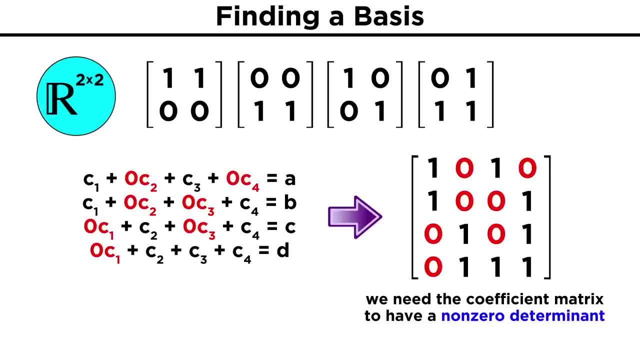 So let's just set up the coefficient matrix, making sure to put zeros where the coefficients are missing in each equation, and then find the determinant of this 4x4 matrix, which won't be too difficult. Considering all the zeros, We end up getting a determinant of one which is indeed not zero. so a solution does exist. 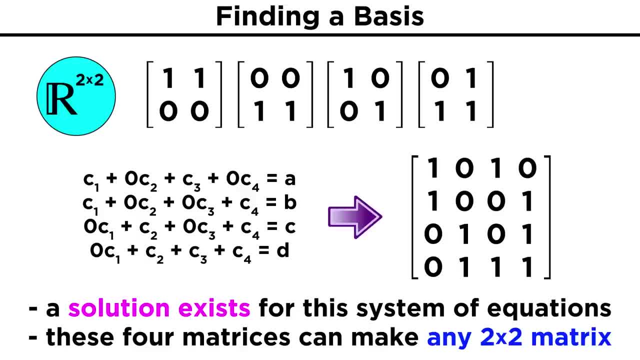 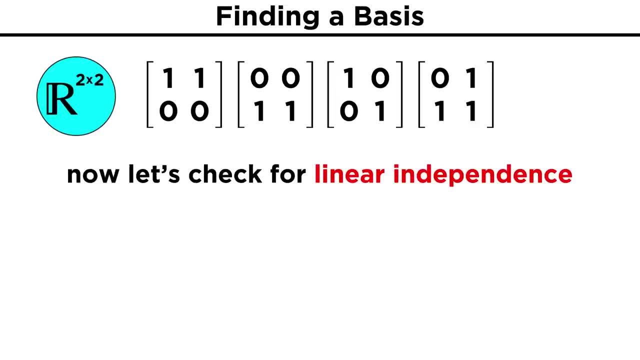 to this system of equations and our matrices can therefore be used to make up any 2x2 matrix. This means that our matrices span are 2x2.. Next we must check for linear independence. Let's take the same linear combination we just used and set it equal to a matrix full of zeros. 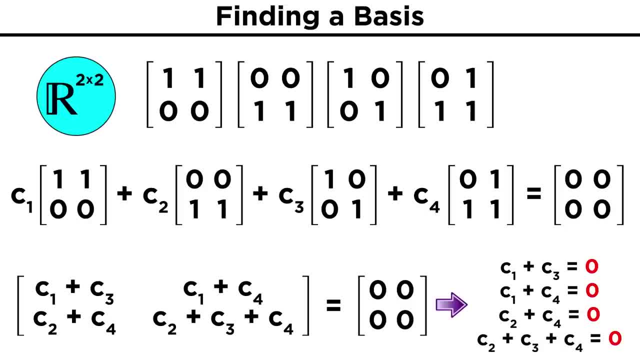 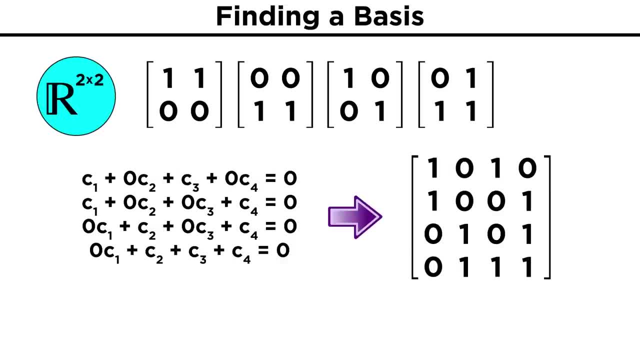 We end up with the same equations as before, but with all the values on the right-hand side being equal to zero. We could solve these equations a few ways, but let's go ahead and use elementary row operations to get the coefficient matrix into row echelon form. 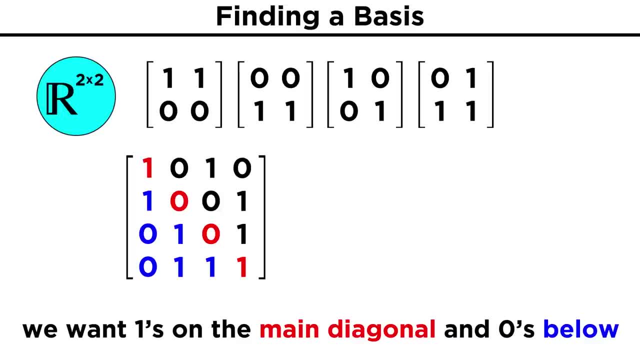 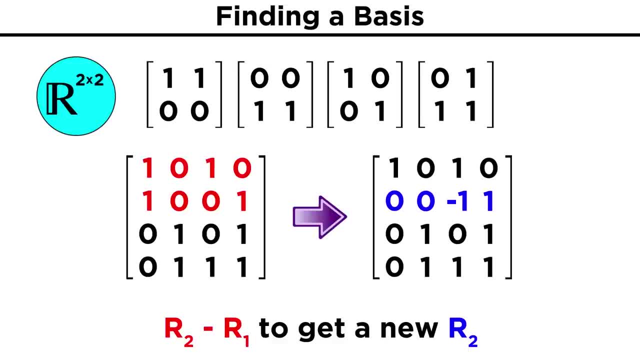 Let's start off by taking the second row and subtracting the first from it Next to get ones where we want them. let's switch rows two and three. Now we can multiply the third row by negative one to get positive one here. Next, to get rid of this one in the second column of the fourth row, let's subtract. 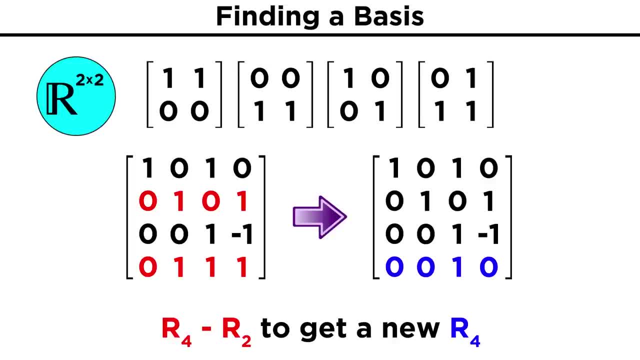 the second row from the fourth row. Next, to get rid of this one in the third column of the fourth row, let's subtract the third row from the fourth row And this will leave us in row echelon form. We are left with no free variables. in this form, all the diagonals have a leading one. 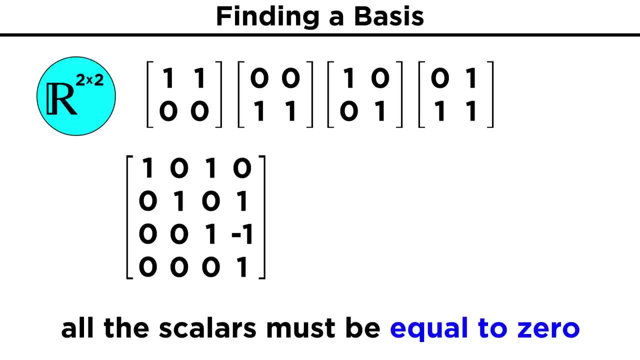 This means the only solution is all the scalars being equal to zero, which we could check by writing the matrix in equation form. once again, We can now write the matrix in equation form Using this last equation: C4 must be equal to zero, and once we plug that into the equation, 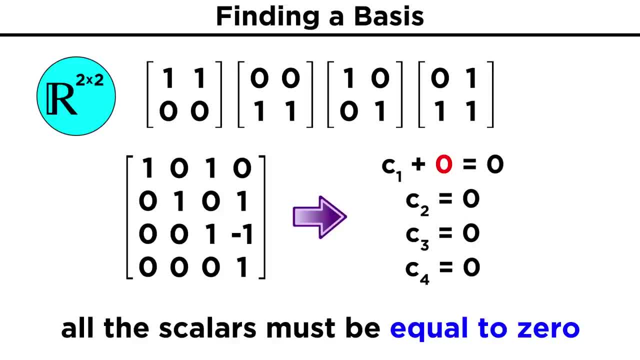 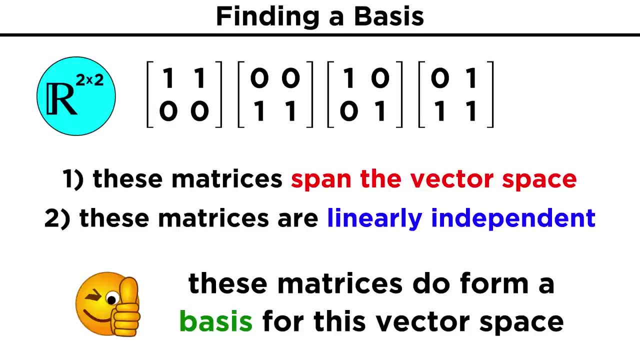 above to get C3, and continue from there to get the other two. we end up with all zero scalars. Thus our matrices are linearly independent. We have verified both conditions for these matrices to be considered a basis for R2x2.. 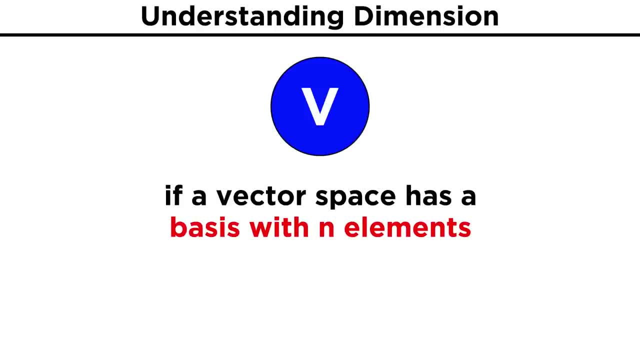 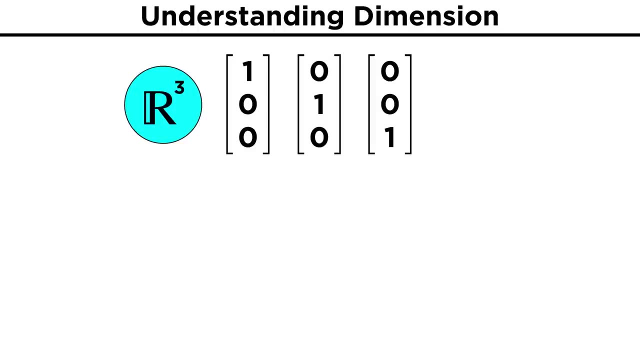 Before we wrap things up, we should go over one more definition. If a vector space, V, has a basis made of n elements, then the vector space is said to have dimension n. Taking our two examples from this lesson, we saw that R3 had a basis made of three vectors. 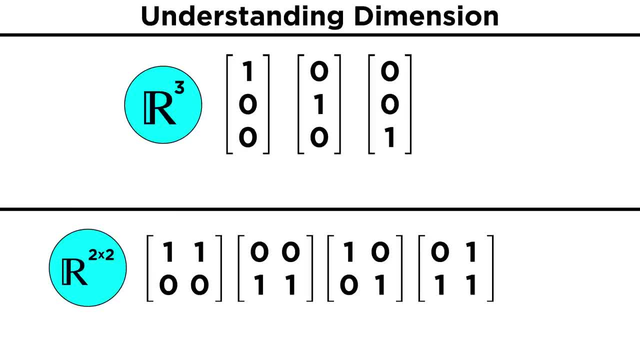 and R2x2 had a basis made of four matrices. We can then say that R3 has dimension three and R2x2 has dimension four. We can then say that R3 has dimension three and R2x2 has dimension four. 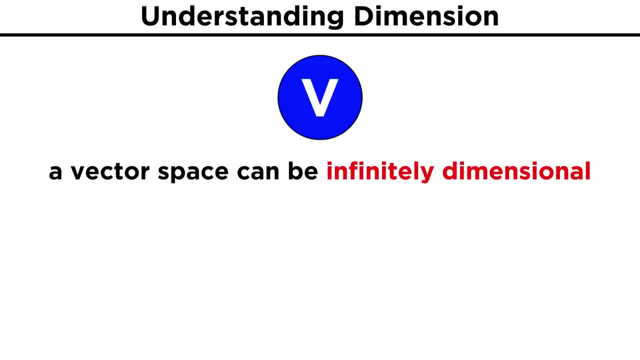 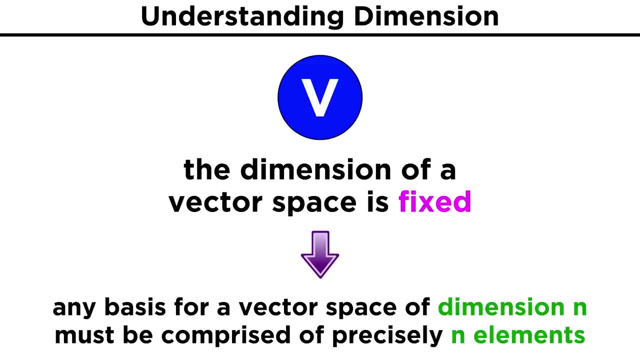 Upon these examples, it is possible for vector spaces to be infinitely dimensional. and we also say that the set which contains only the zero vector element has dimension zero. The dimension of a vector space is fixed. so no matter what basis we end up using for